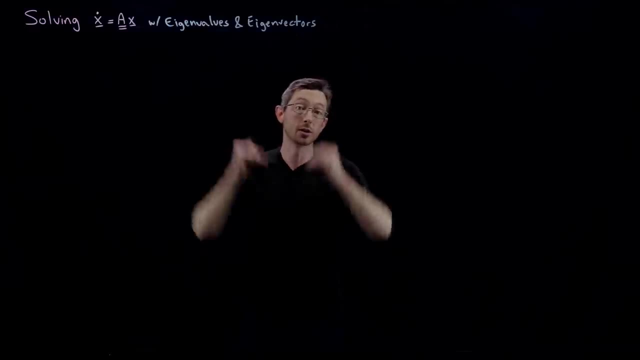 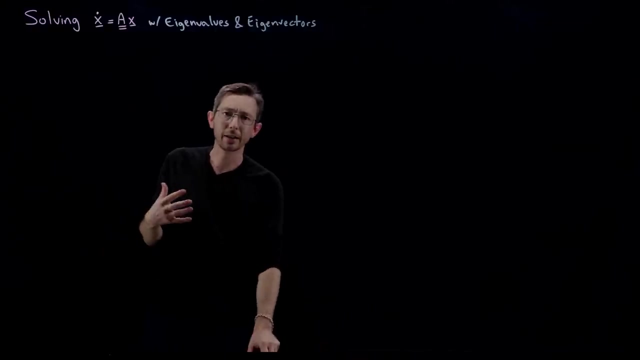 going to end on kind of deriving from scratch the equation from which we obtain eigenvalues and eigenvectors, specifically to solve this system. Okay, so I'm going to write out the objective, I'm going to solve a simple case and then we're going to jump into eigenvalues. 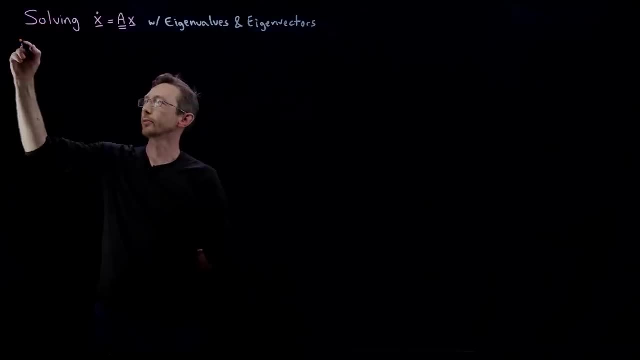 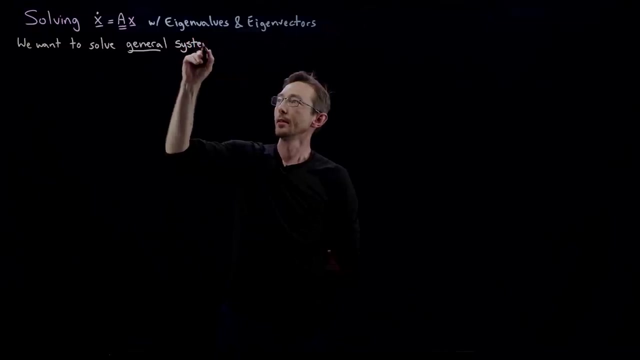 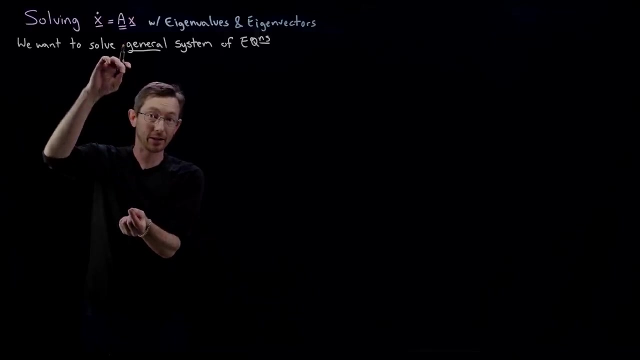 and eigenvectors. So we basically want to solve this system. We want to solve a generic system of equations, a general system of ordinary differential equations. x, dot equals ax system of equations And specifically, x is a vector of states. now 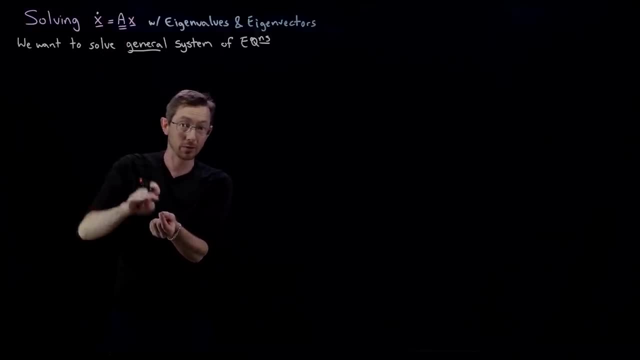 There are multiple, You know x1, x2, x3, x4, multiple components of this vector. x A is a matrix and this is a system of coupled first-order linear ordinary differential equations. First-order because we only have one derivative in time, coupled because presumably these derivatives 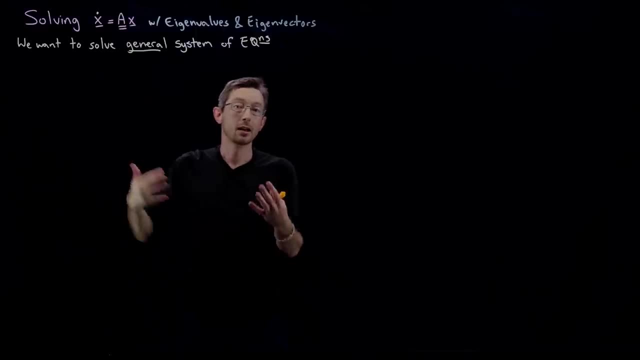 depend on all of the other states in this vector, x and linear, because this derivative x- dot is a linear combination of the states in x. That's literally what a matrix times a vector means. That's a linear combination. Okay, And so what I'm going to do is I'm going to start off with the simplest possible case where this A matrix is diagonal. 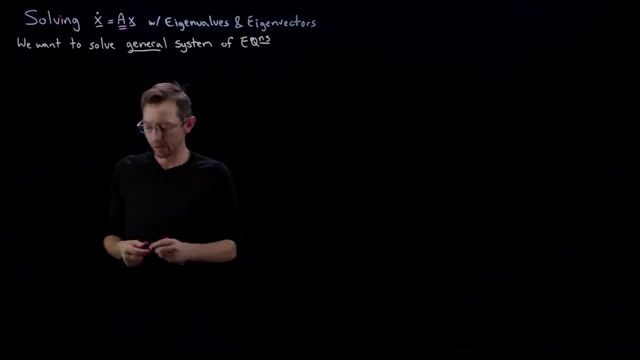 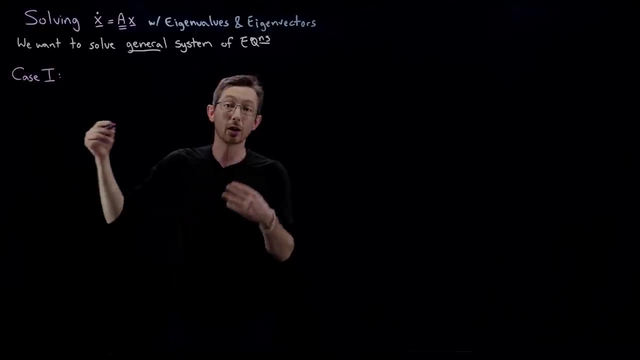 meaning that the dynamics are decoupled, Okay, So kind of case one. case one is where what we have, what we call decoupled dynamics, Decoupled, decoupled, Decoupled, decoupled, Decoupled dynamics. 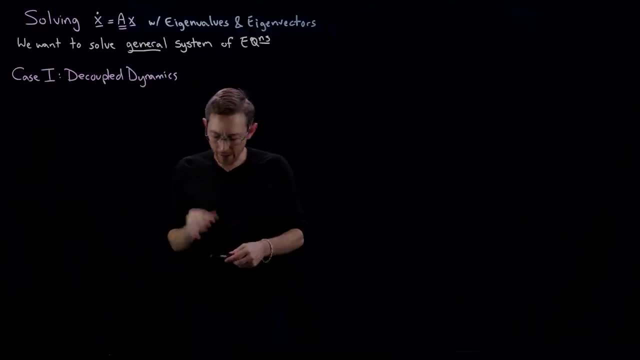 I'll tell you what that means. So remember when we had kind of our first example of a differential equation: x dot equals lambda x. The example we introduced was the population of bunnies, and bunny populations grow exponentially. What I mean by decoupled dynamics is going to be, let's say, that the state x refers to the populations of different animals. 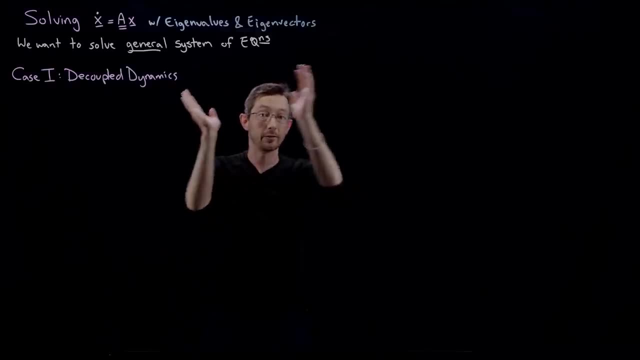 but they are kind of in a zoo, So they're each cordoned off into different zones and so that they don't interact. That's what I mean by decoupled. So we're going to have the populations of, like bunnies and wolves and antelope. 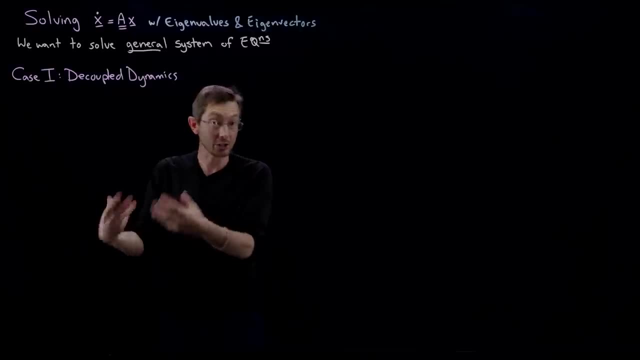 And so I'm going to have a state vector with multiple populations and they're each going to behave linearly, but they're only going to depend on themselves. They're not going to be coupled yet. So I like to call this kind of. you know, my example I think about is different animals. 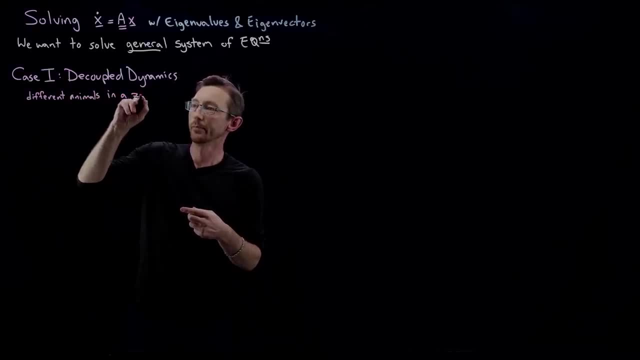 So I'm going to have a zoo in a zoo, and it's a zoo that's big enough where they can grow exponentially. It's kind of like a Hilbert's Zoo or something like that. Okay, so the populations are separate. That's the key thing is that the populations are separate. 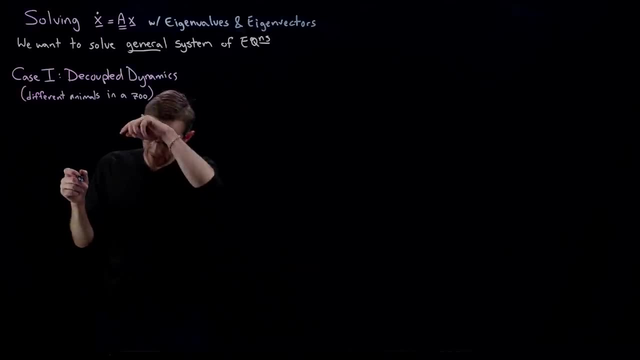 And so I'm going to write down this differential equation. So we have, let's say, our state. vector x has a bunch of components: x1,, x2,, dot, dot, dot, all the way to xn. Let's say, I have n. 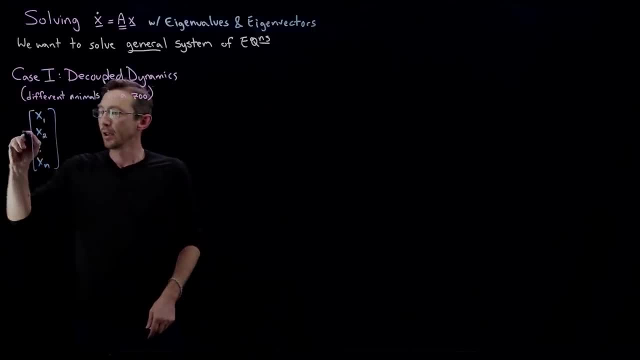 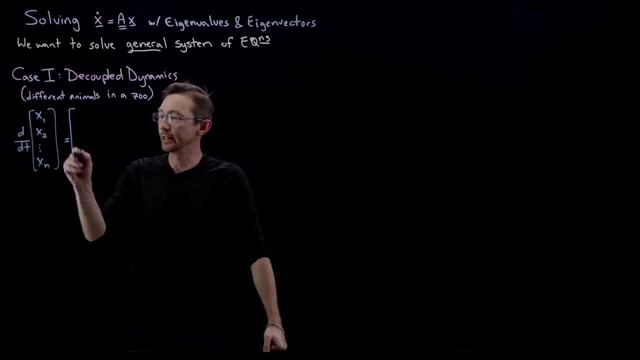 Animals in n different zones in this zoo, And I'm taking d d t of this state vector that's just this, is just x dot, where x is a big vector containing all of these components And we're going to say that this equals, in the case of decoupled dynamics. 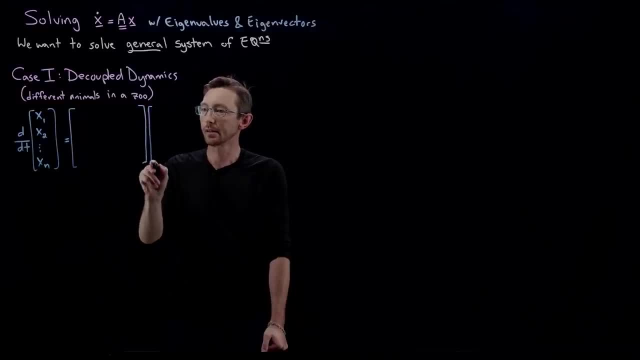 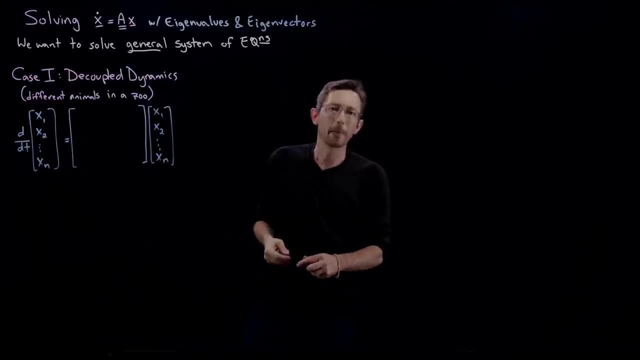 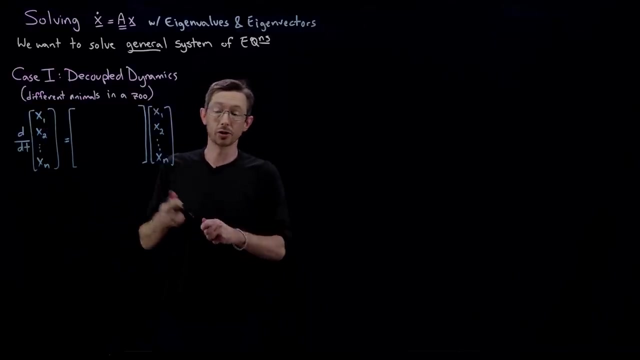 this is again a matrix A times x1, x2, dot, dot, dot, xn. But now what we're going to have is that this is going to be a diagonal matrix, So x1, dot is only going to be a function of x1.. 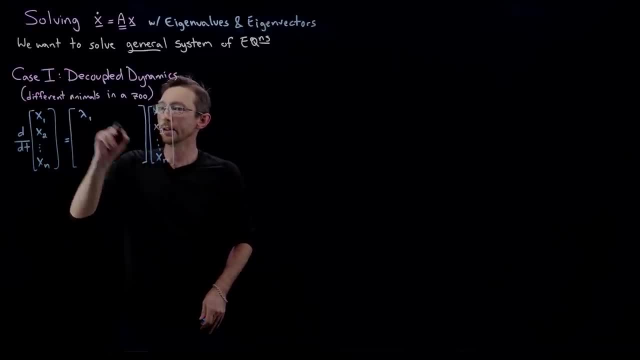 We're going to call that? let's say, you know, lambda, 1,, 0,, dot, dot, dot, 0.. The second animal, let's say x1,, our bunny population. Okay, x2,. let's call that our wolves. 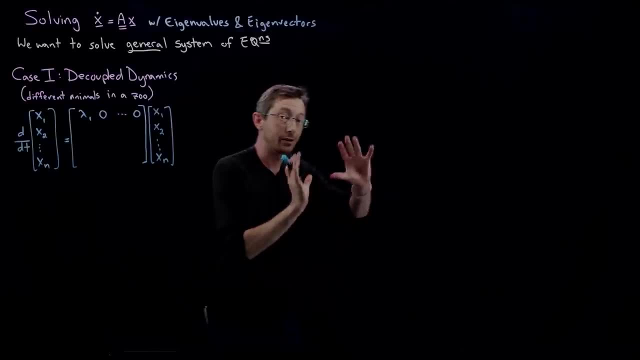 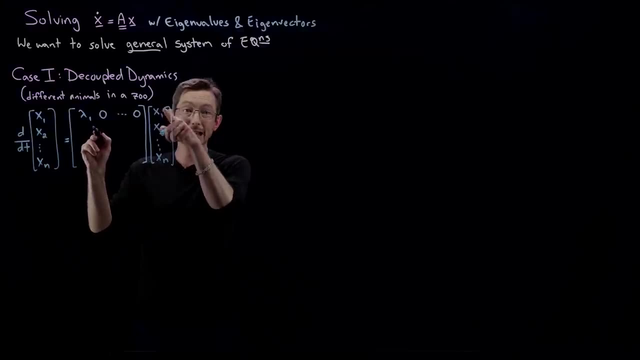 x2, dot is only going to be a function of x2 because they live in their own you know room in this big zoo. So they actually are not, you know, in the zoo. They're not interacting with the bunnies, so they have no influence. x1 has no influence on x2.. 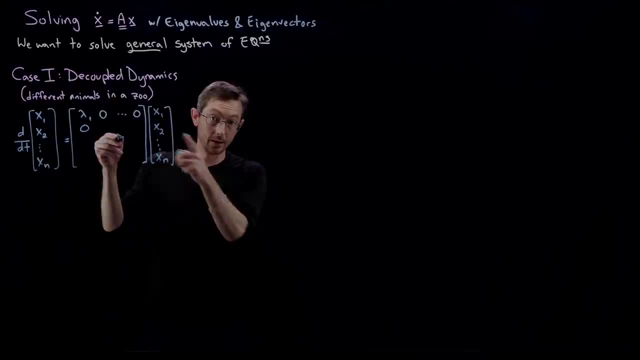 x2, dot is only equal to a number times x2.. We're going to call that number lambda 2.. So x2, dot equals lambda 2 x2.. And that's the only. these are decoupled. so you know, the wolves are alone, the bunnies are alone. dot, dot, dot. 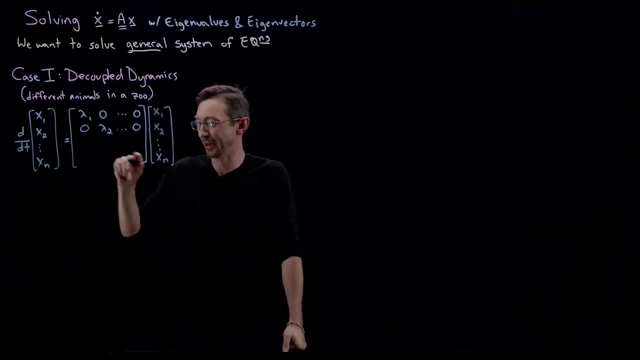 It's very lonely. Actually, I think they're fine with you know all the bunnies together And then kind of every term is like this: And now the xn dynamics, the nth population, whatever only depends on the xn population, with this lambda n proportionality. 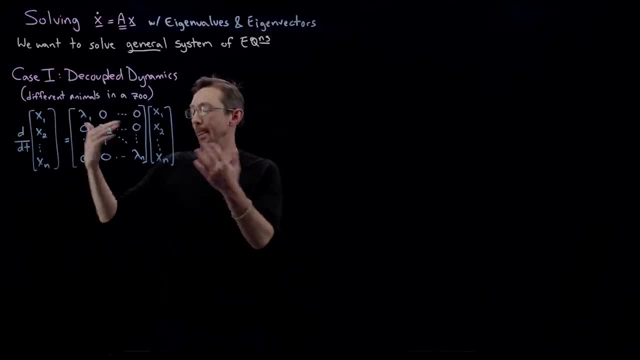 So this is really, really simple. In some case, I didn't even need to write this as a system of differential equations in a matrix form. I could have literally just written this as so, before I forget, I'm going to call this matrix d, because it's diacritic. So, before I forget, I'm going to call this matrix d because it's diacritic. So, before I forget, I'm going to call this matrix d because it's diacritic And then it's going to become a diagonal and decoupled okay. 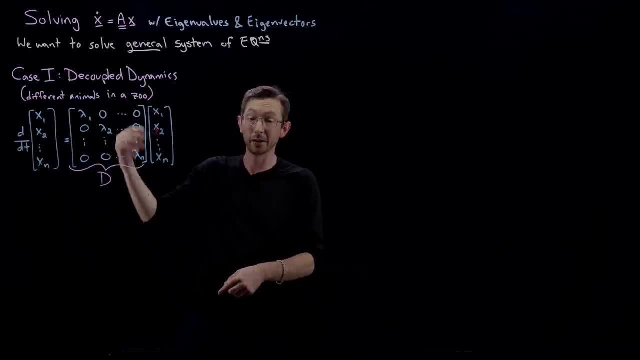 So this is a special case of an A matrix where it's diagonal and decoupled. I didn't even have to write it like this. I could have literally just written down: you know, x1 dot equals lambda 1, x1.. 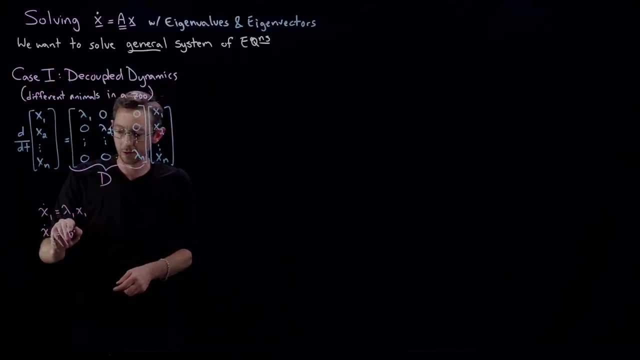 So this is a special case of an A matrix where it's diagonal and decoupled: X2, dot equals lambda 2, x2,, dot, dot, dot, Xn, dot equals lambda n, xn. And, and of course we already know this employee. 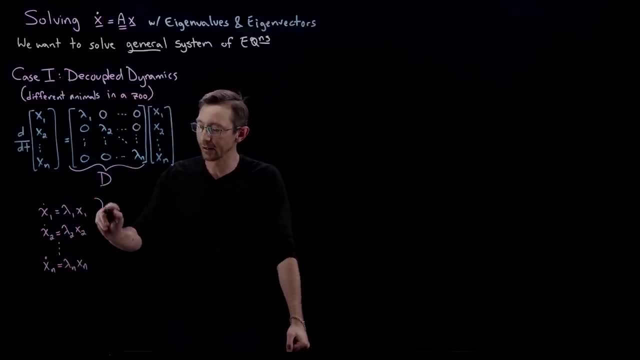 And he did". Okay, And solution of this? we can just solve them each independently. We could say that x1 at time t is e to the lambda 1 t times x1, my initial condition: x1 naught and x2 at time t is equal. 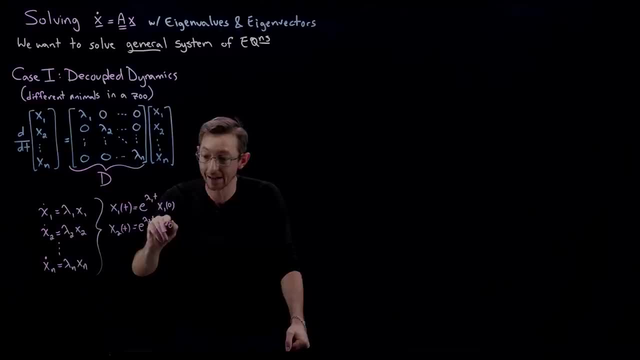 to e to the lambda 2 t times that initial wolf population. x2 naught all the way down to xn. at time t equals e to the lambda n t times xn naught the initial population of that nth animal population. And so these are really easy Because my dynamics are decoupled. 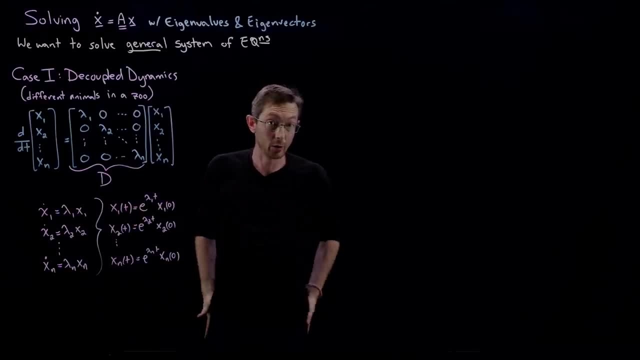 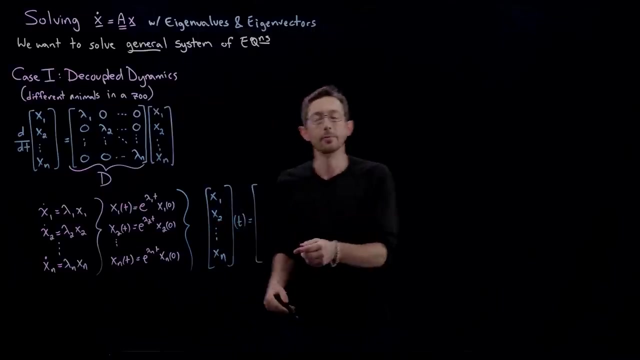 it's almost trivial for me to solve the system of equations And if I like I can write this solution again in matrix form. I can just say: you know, this is x1,, x2,, x2,, dot, dot, dot, xn, this big vector x, at time t is equal to, and now I have a diagonal. 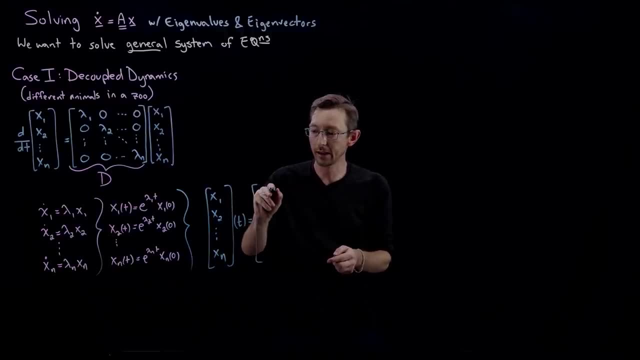 matrix of exponentials. I have e to the lambda 1 t 0, dot, dot, dot 0.. I have 0 e to the lambda 2 t dot, dot, dot 0.. So this should be pretty, you know, intuitive at this point, 0,, 0 e to the. 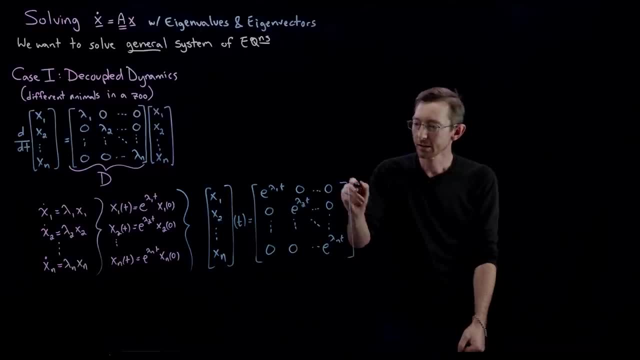 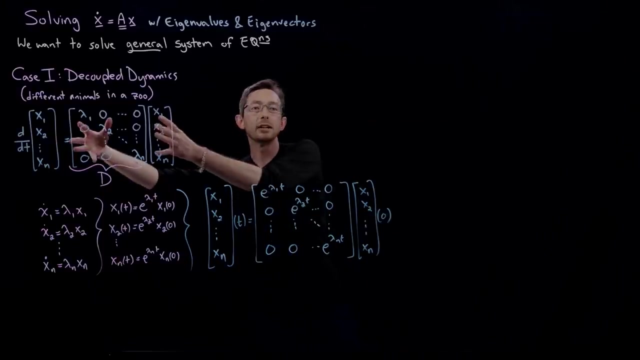 lambda n t times, my initial conditions times, you know, x1, x2,, dot, dot, dot, xn. this vector evaluated at time 0.. Okay, and so this is really really simple. This, if this matrix here was d. 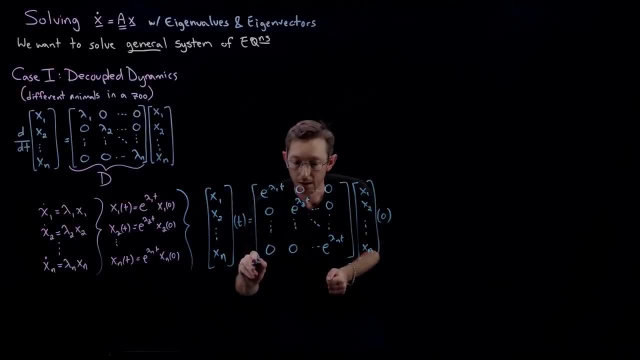 a diagonal matrix, then this matrix here is e to the diagonal matrix t. Okay, it's literally a diagonal matrix. It's not a diagonal matrix, It's a diagonal matrix. It's a diagonal matrix Where I exponentiate all of the diagonal elements times t. this is e to the d t I haven't defined. 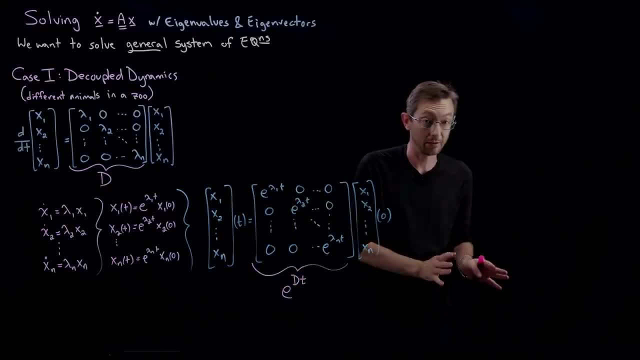 what a matrix exponential is. yet I'll define that in a couple of lectures. It's really easy. You literally take the Taylor series- for you know e to the x and you just plug in a matrix for x and you work it out. That's how you take matrix exponentials and this is what you get for. 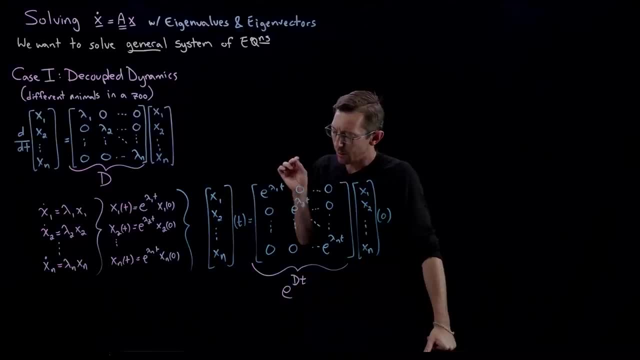 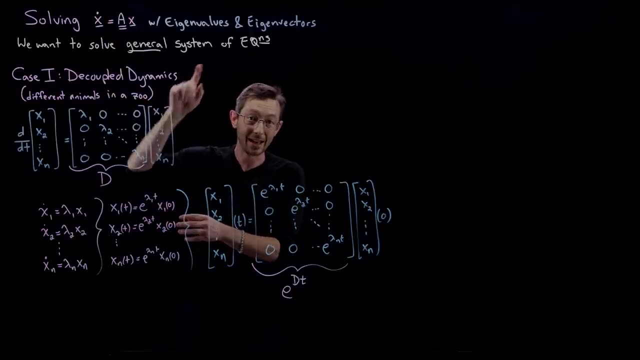 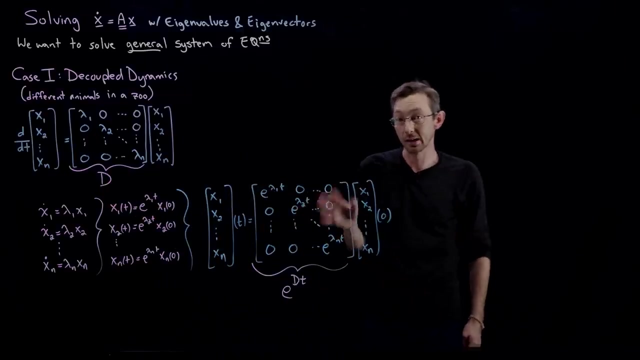 decoupled dynamics. Okay, so this is really really, really easy. I'm going to show you a little bit of how easy it is to solve my system of equations. x dot equals ax if a is a diagonal matrix, d. Good, So I hope I've convinced you that that's really really easy. Okay, this is the full. 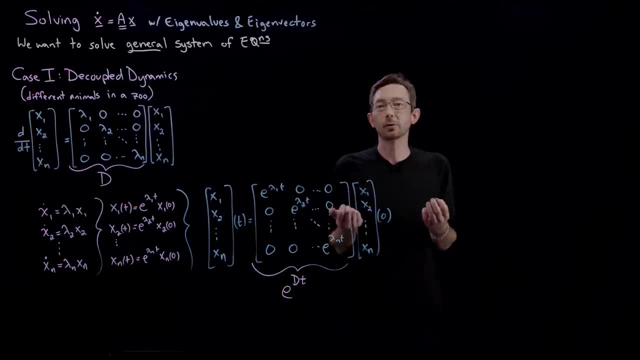 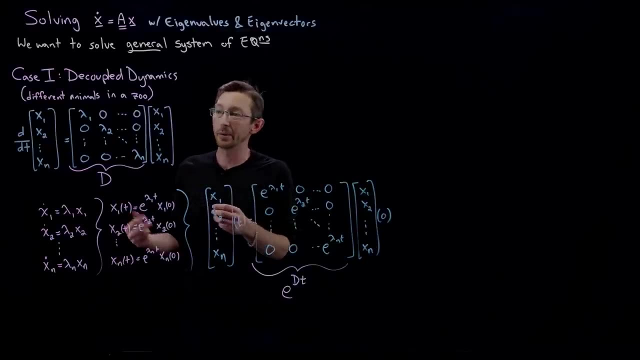 solution. But most of the systems we deal with in the real world are not going to be nice and diagonal like this. You know you're not going to be dealing with animals in a zoo. You're going to be dealing with the populations of bunnies and wolves and antelope in the wild, and they're not. 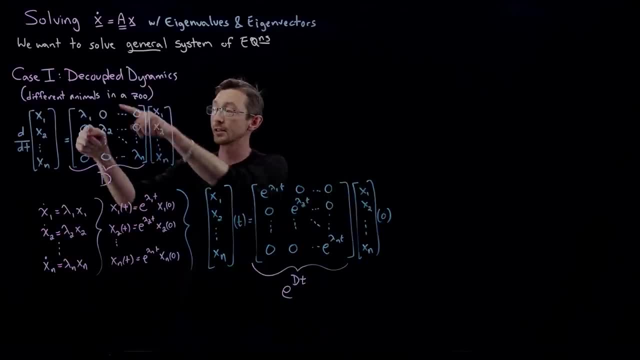 going to be separated. They're going to be separated. They're going to be separated. They're going to be interacting with each other. So there's going to be cross terms in this matrix and, in general, a is not going to be diagonal. It's going to be a full, gnarly matrix and it's 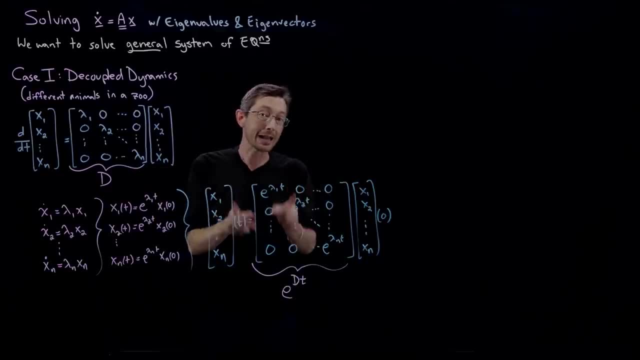 not going to be easy to solve it like this. Okay, and so that's where eigenvalues and eigenvectors are going to come in. What we're going to try to do is we are going to try to find a coordinate transformation that turns this system into a diagonal decoupled system. I'm going to erase 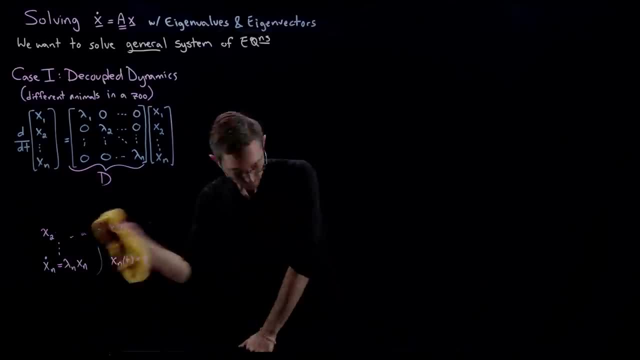 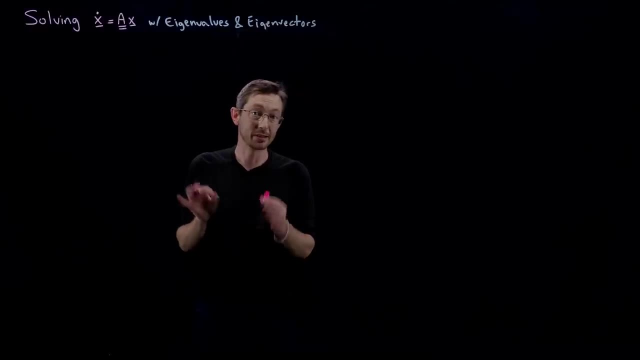 this And then write that out One second. Okay, so we now know that it's easy to solve these matrix systems of equations if the matrix A, relating all of my derivatives to all of my states, is diagonal and decoupled. So now the 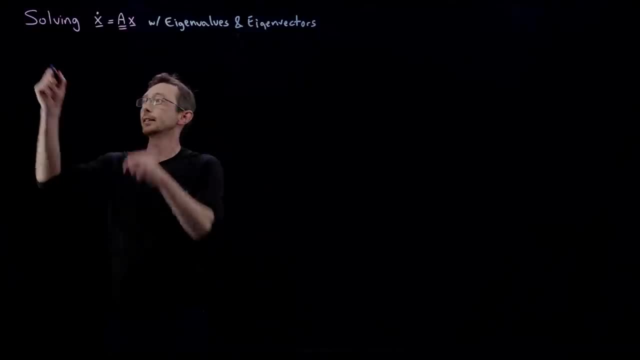 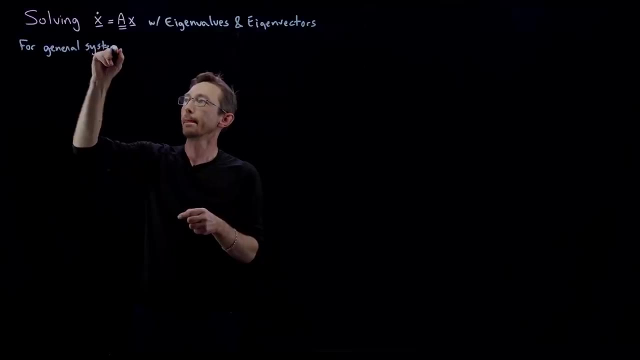 objective here is going to be, for this generic system, for a general system, for a general system, X dot equals AX- what we're going to try to do. we want a change of coordinates, We want a new coordinate system or a change of coordinates, A change of coordinates, And I'm going to write: 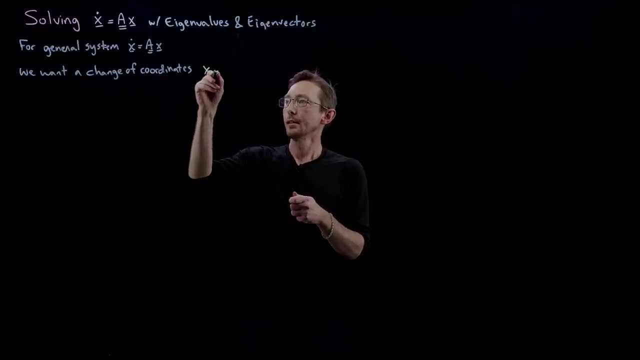 this, as X equals T times Z, So T is going to be a matrix. Now Z is an invertible matrix, a matrix that has non-zero determinants, So you can compute its inverse. so I can go from X to Z or Z to. 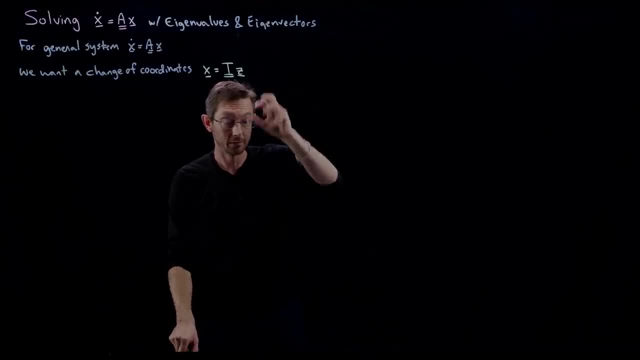 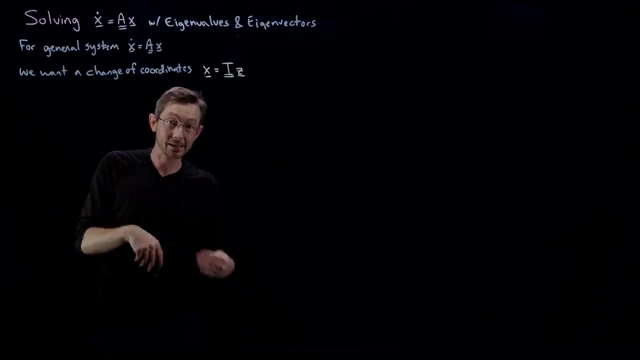 X by multiplying by the matrix T or its inverse. So I want a change of coordinates into a new coordinate system Z that diagonalizes my Oderrnary differential equation, that diagonalizes my OD. That's not a very easily or quickly way to do it. 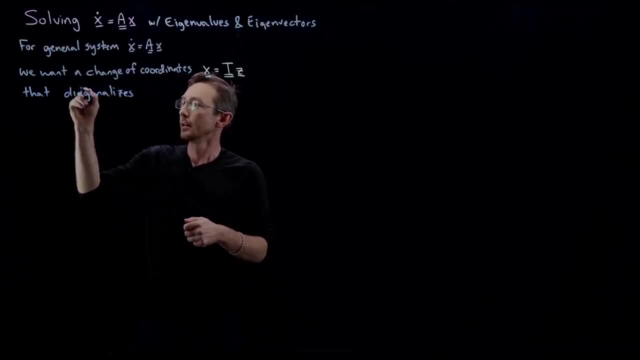 Okay. so in fact let's call each of these up and go back to them. dig- Okay, so include at the end all of youranta in every area within this permanence and dig the new coordinate system in the order M to the soonest chart back so that you're only left with 1 over the next one. 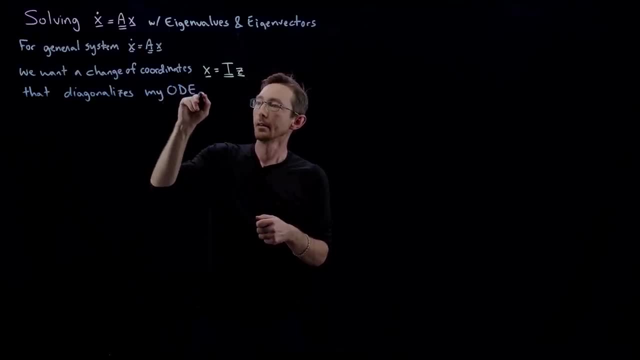 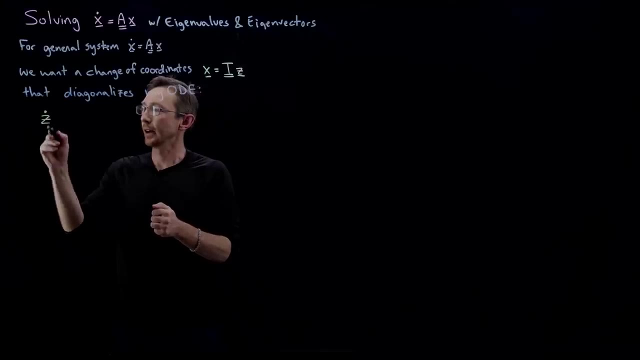 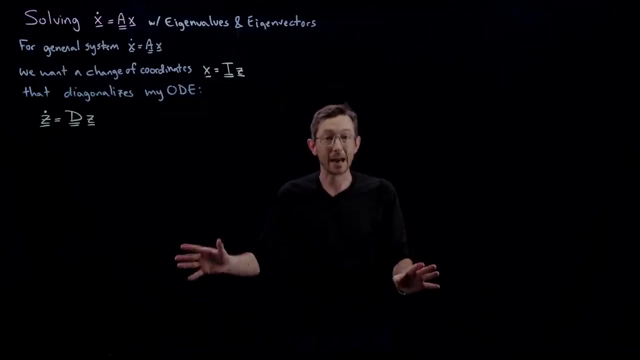 That's just the L. consider if the matrix P is the daytime ON or the next day before the end. on the date, my ODE. Specifically what I want in this Z coordinate system, I want Z dot to equal a diagonal decoupled matrix times Z. okay, That's my entire objective. now, If I have a generic system, 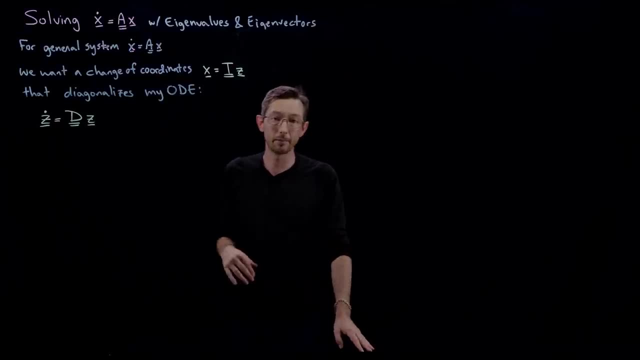 if someone hands me a system and they say: hey, Steve, can you model this system? I'm going to first try to find a coordinate transformation T that goes back and forth from, you know, from X coordinates into a Z coordinate system, where, in this coordinate system, my dynamics are decoupled. 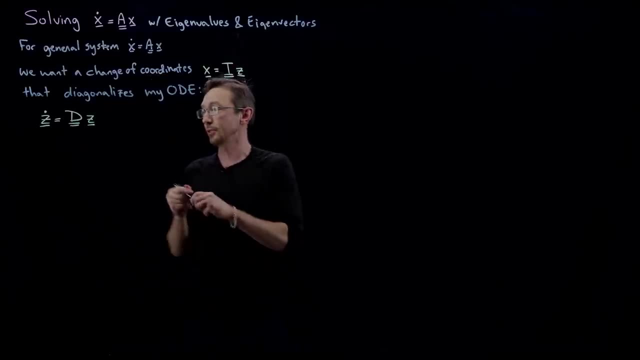 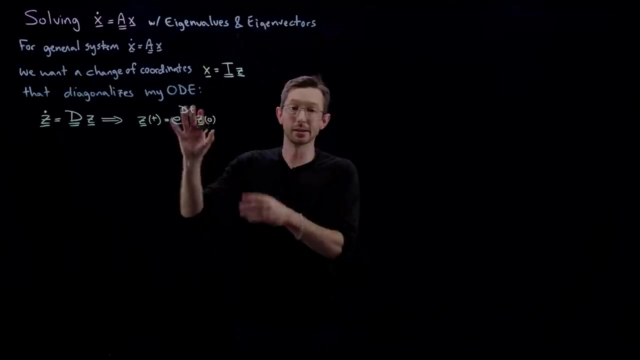 and diagonal, Because here I could easily solve this. We know how to solve this. Z as a function of time is E to the matrix D times, time times, my initial conditions. I know how to solve this. This is easy to solve, We. just. 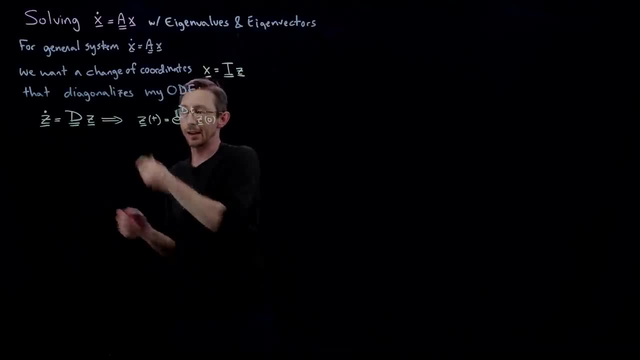 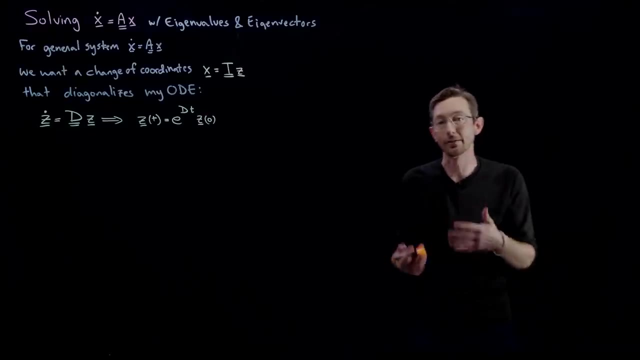 did it. So now I'm going to try to find this coordinate transformation that diagonalizes my system. okay, And specifically, we're going to do this and we're going to derive the eigenvalue and eigenvector equation. So I'm going to take the time derivative of both sides of this thing. 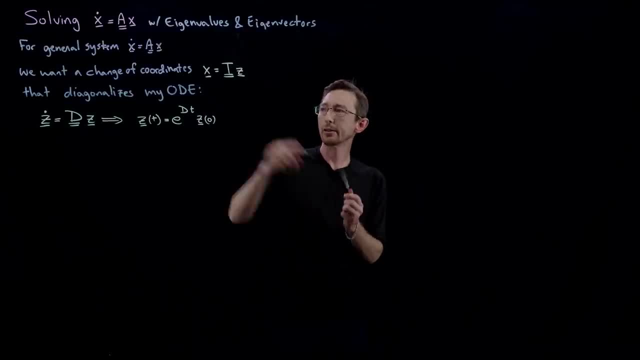 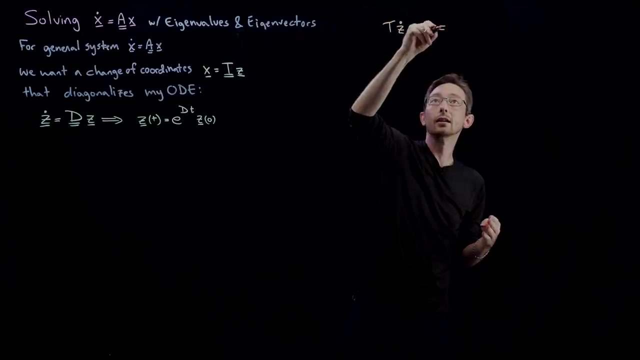 Maybe I'll go orange here for a minute. So I'm going to take the time derivative of both sides and I'm going to take T Z dot. that equals X dot and X dot equals A X. So that equals A X And so that implies that T Z dot equals A X. 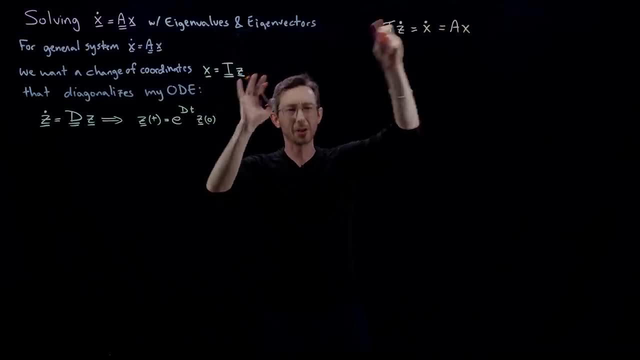 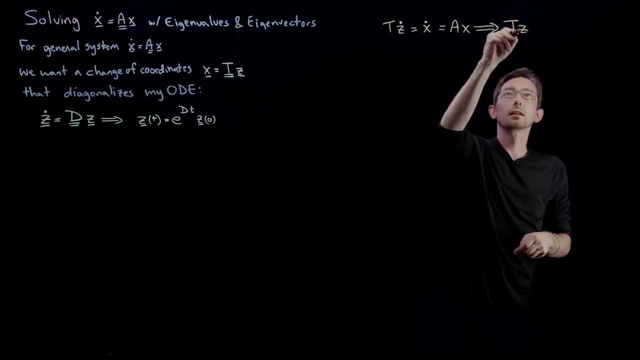 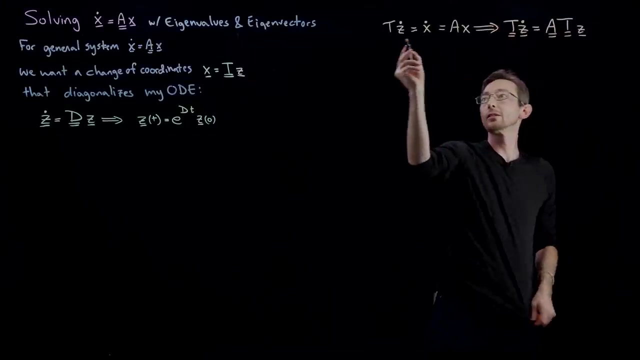 And specifically X equals T Z. So here I can plug in. I'm trying to get an equation for Z. So I can basically say that T Z dot equals A times X, and that's A times T times Z. This equals A times T times Z, And now I'll remember to put all of these matrices and vectors. So big capital. 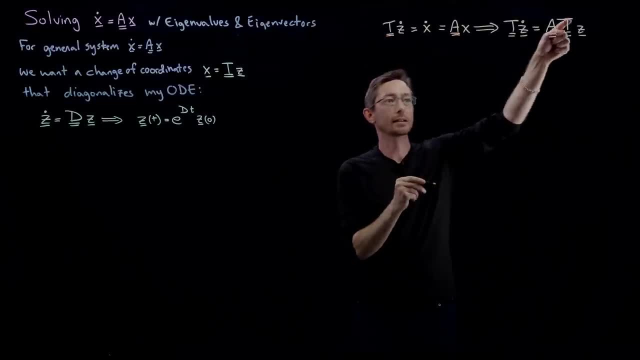 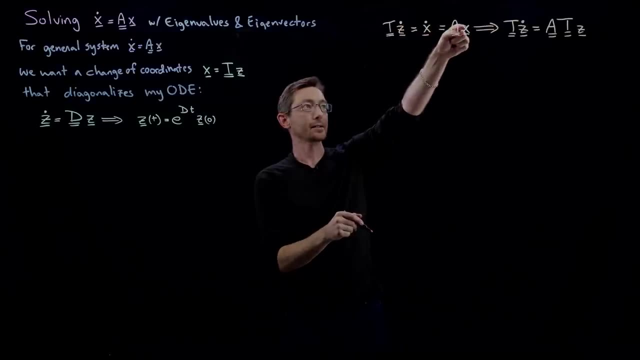 letters generally I use to mean matrices. So A and T are matrices, Z and X are vectors. okay, That's the state of my system. X and Z is the state of my system in some different coordinate system. okay, And I'll tell you what I mean by a different coordinate system in a minute. Okay, so now this. 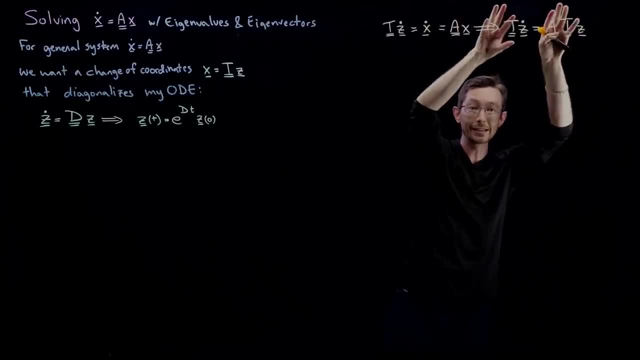 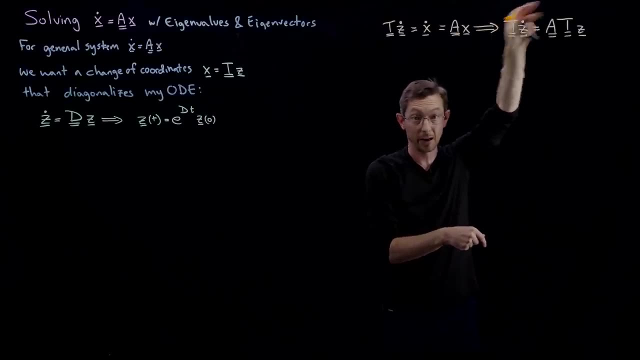 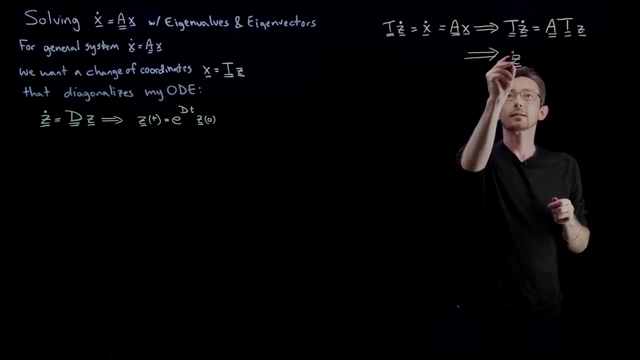 is starting to get somewhere. Now we have to figure out how to solve this. So I'm going to have a differential equation only in Z, but I have this pesky T out here, So I'm going to try to invert this T and multiply on both sides by that. So that gives me Z. dot equals T, inverse A T times. 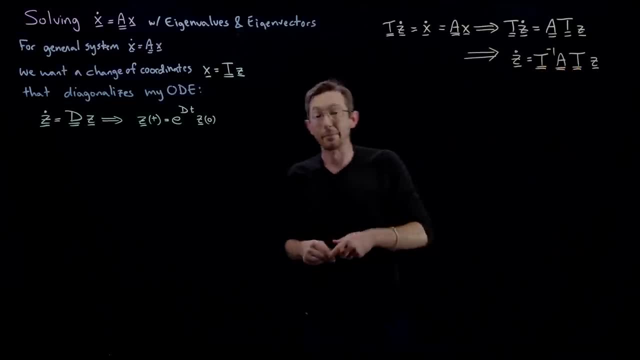 Z. And remember, I'm specifically trying to find this coordinate, I'm trying to find this matrix T. That's what I mean by a coordinate transformation. It's just a matrix T. Linear coordinate transformations are matrix multiplication. That's what linear algebra tells us, And so 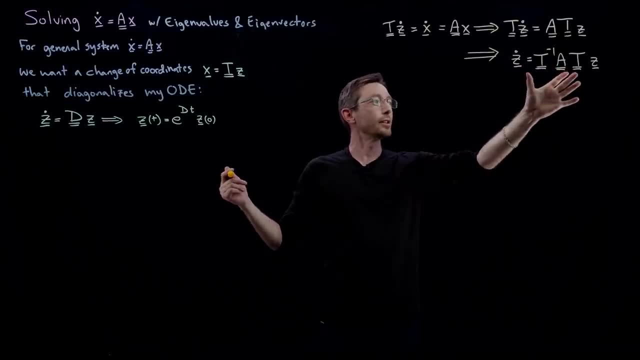 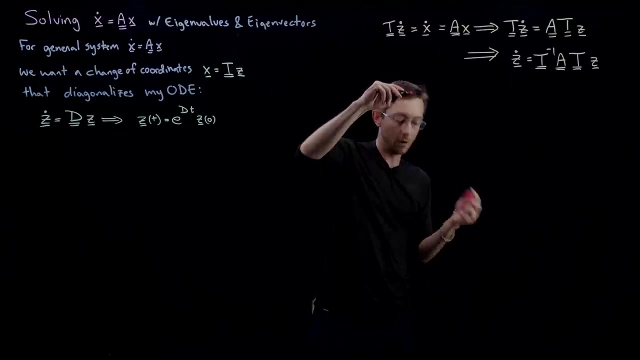 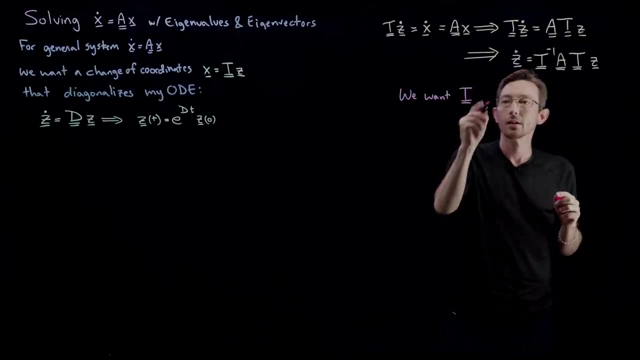 specifically, I'm trying to find a T matrix so that this quantity here is a diagonal matrix, So that Z dot equals this stuff here is diagonal times Z And so specifically, like we can write that, So I need thisどうだぜ, So I'll hold this right and tie this, So I already know it's going to. 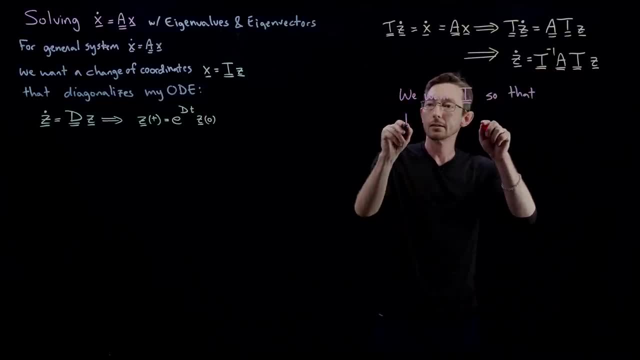 multiply right there, And I'm going to divide it by 2xn, so I can just add the 10 times to catering so that we can see theачesi in this column. okay, So that's what we're going to do with this matrix T. 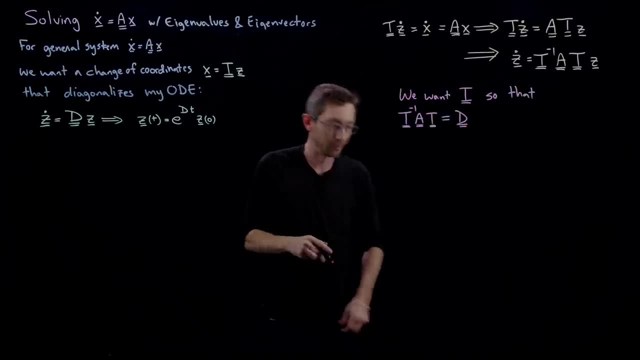 And that's times T, It's any scale, like you know, thinking about a regular item like division of assets in this washing machine. If that's the case, that's the first thing we're going to do is change the Hebrew, So we just orange off this escriblings that came up in the exercise. So we're going to Women's. 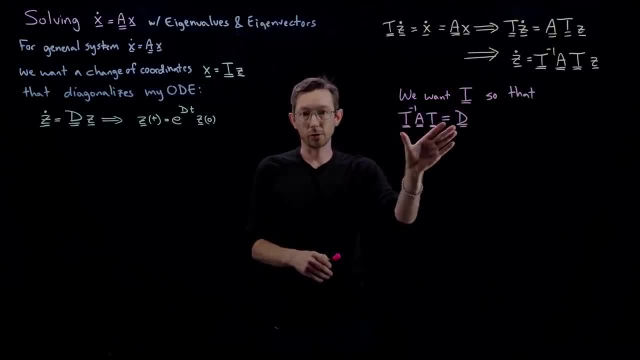 Law class is a little bit more complicated, And then we'll go through this on our regular course because we're getting way too much knowing so much together. So what I'm going to do, equipped with: So we want a T, so that this is true. 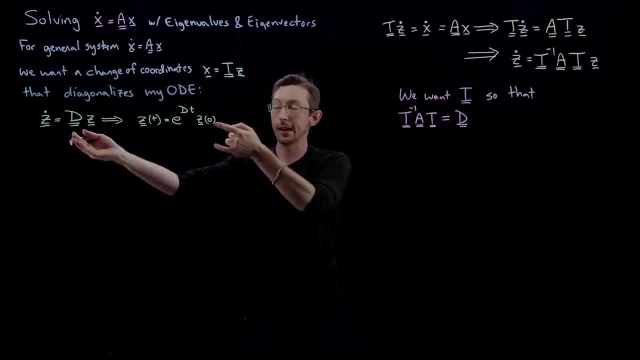 We had this system, We want to find a coordinate transformation that diagonalizes our dynamics. And if we had a T, so that T inverse AT equals a diagonal matrix? we've done it, Okay, And so the last step. this is actually like very, very simple. 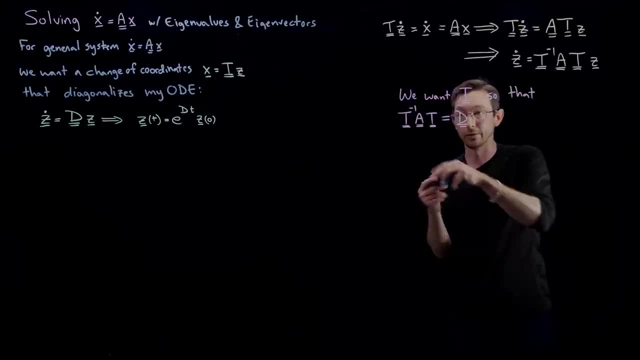 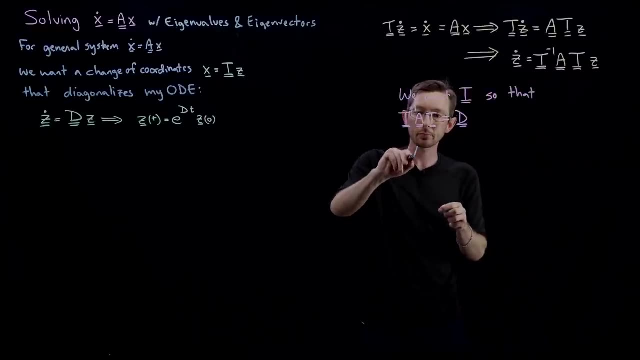 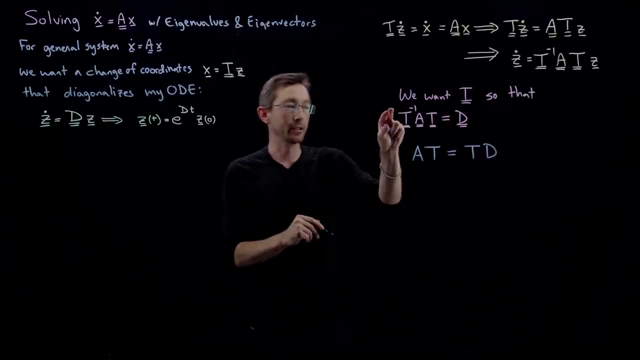 The last step here is: I'm just going to multiply both sides again on the left by T to kill this T inverse, And so that is going to give me AT equals TD. I multiplied the left by T on both sides so I get AT equals TD. 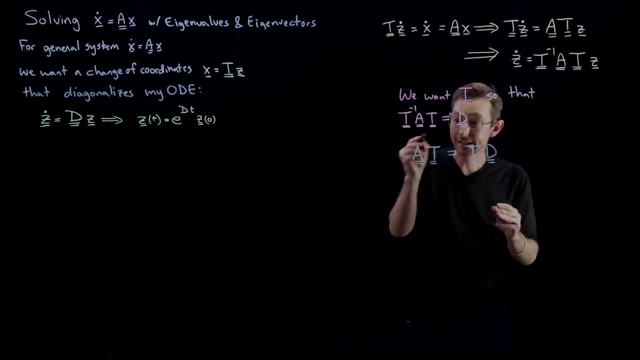 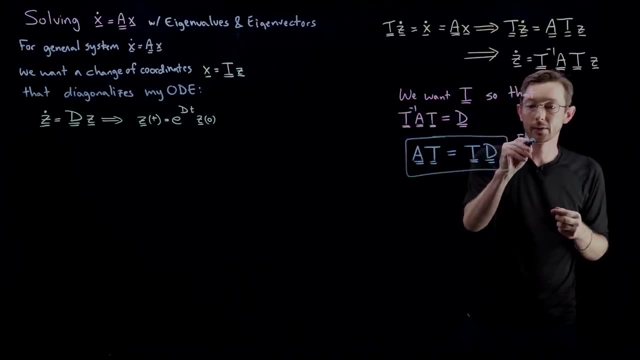 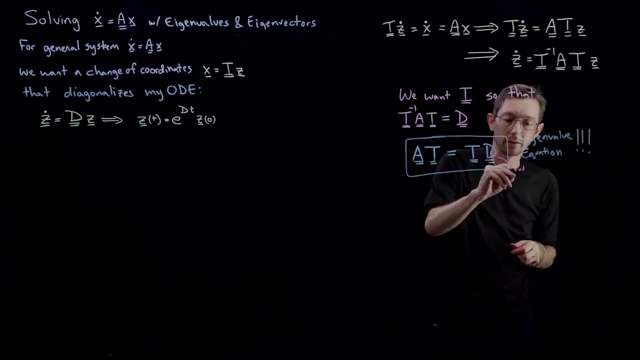 These are matrices. This is the eigenvalue and eigenvector equation. This is the eigenvalue equation. Eigenvalue Equation. I'm going to put some big exclamation marks because this is a huge deal. Literally. the diagonal elements of D, the diagonal elements of D are the eigenvalues. eigenvalues of A. 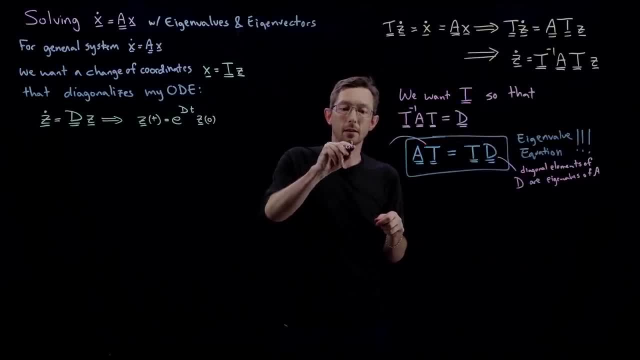 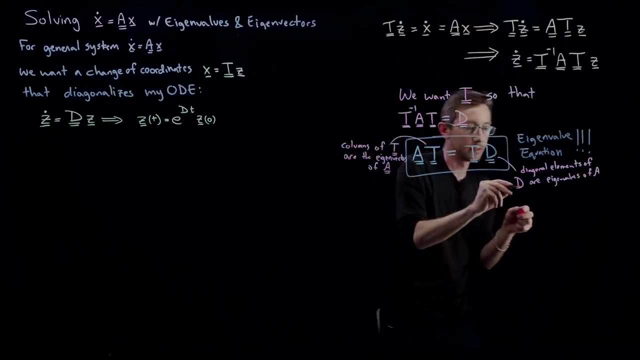 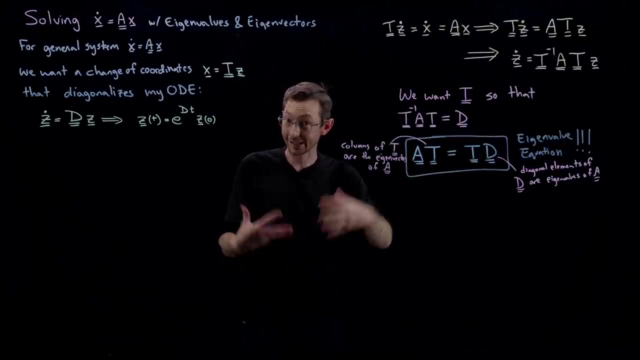 And the columns. The columns of T are the eigenvectors of A. Okay, D is a matrix, A is a matrix, So I haven't shown you how to solve for T and D. That's a whole other lecture. I'm going to do that next. 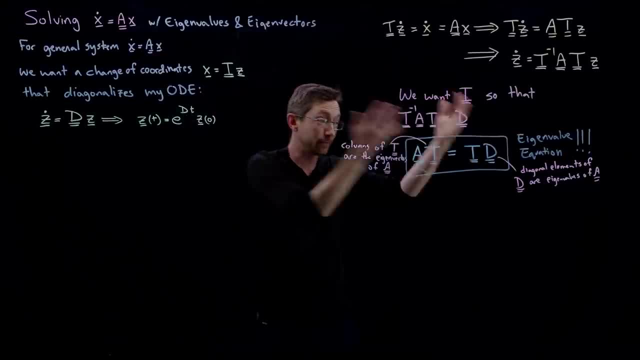 We're going to show how, for a specific A matrix, we can find these eigenvalues in D and the eigenvectors: We can find these eigenvectors in T. but this is the equation, the equation that I'm solving for T, so that my dynamics become diagonal. those T are the eigenvectors of A. 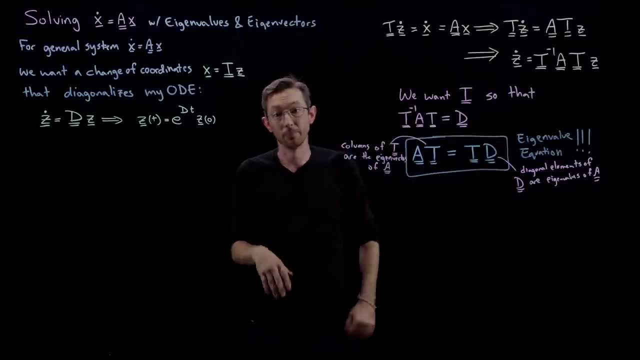 That's exactly what this means. This is the eigenvalue- eigenvector equation. So for me I always found it very counterintuitive that you take a linear algebra class and they write down all this abstract kind of algebra and they write down here's what an eigenvalue and eigenvector is, without motivating it. 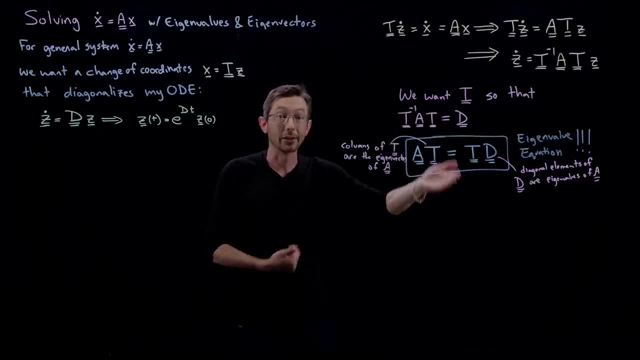 For me. this is why we care about eigenvalues and eigenvectors in the first place. This is why I care about eigenvalues and eigenvectors, because eigenvectors of a matrix change, or a change of coordinates so that it becomes diagonal. 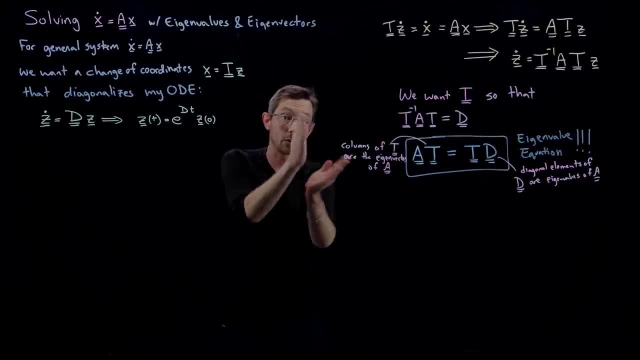 These eigenvectors provide a change of coordinates. In these eigenvector coordinates my dynamics are diagonal. That's huge. That means I can solve any linear system of equations. Okay, So I'm almost done. I think what I'm going to do now is I'm literally. 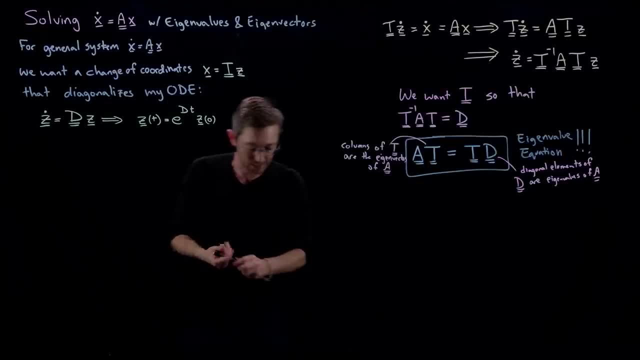 I'm literally going to draw a picture of this for you. So I'm going to say I'm going to draw a picture of this eigenvalue equation and then I'm going to end this lecture And in the next lecture we're going to figure out how do you compute these things and then how do you use these Ts and Ds specifically to solve this equation and then to go back and write it in terms of my original X coordinates, which is where I probably measured things and where I actually care about things. 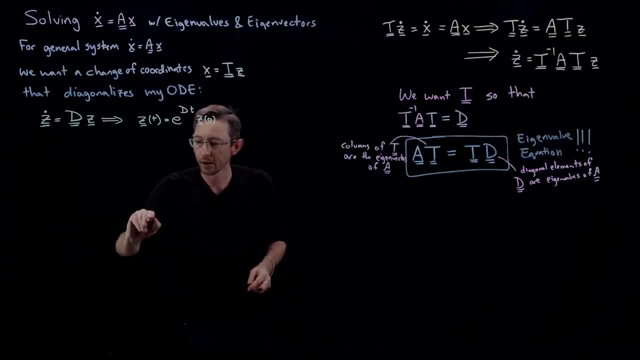 Okay, So I have my A matrix here. I'm just going to draw it as a big square matrix. It's an N by N matrix. Okay, That's A. This T matrix has columns, you know, T1,, T2,, dot, dot, dot, all the way up to TN. 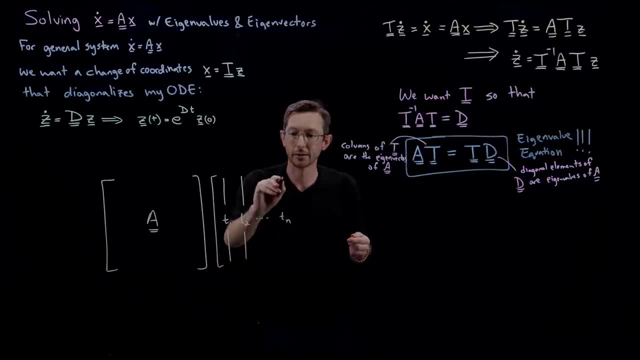 These are column vectors where each column vector is an eigenvector of A, And this is equaling: Now I may be Drew this just a tiny, tiny, tiny bit too tall. That's going to be a problem. Okay, These are the eigenvectors of A. 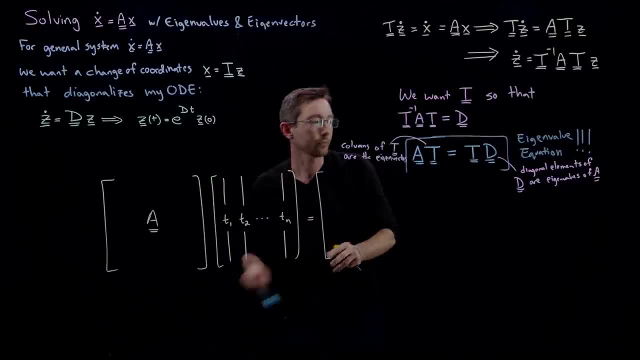 Let's give myself a little more room here. So A times T equals T times D. So this is going to equal again T1, T2, dot, dot, dot all the way up to TN. This is again my T matrix. 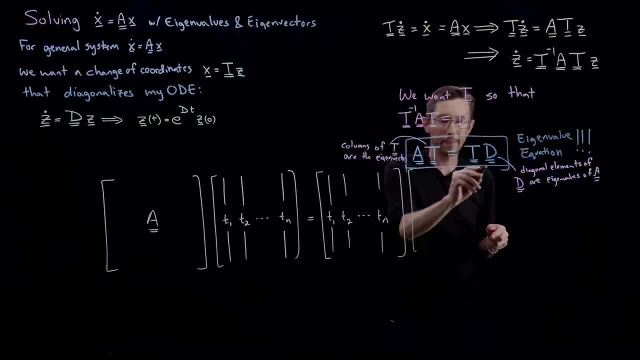 Times D, my diagonal matrix. Okay, And my diagonal matrix again just had these lambdas, these eigenvalues. Sometimes in my notes I call them D1, D2, D3.. Here I'm just going to call them lambda 1, lambda 2.. 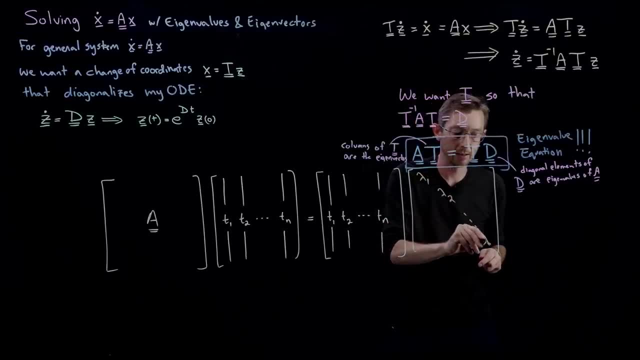 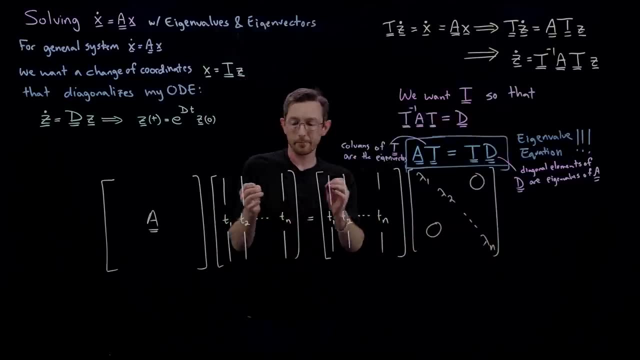 Lambda 1,, lambda 2, dot, dot, dot, lambda N, Zeros everywhere else. And here's what I want to point out Is that, If I take this A column of, So if I want to multiply this matrix by this matrix, 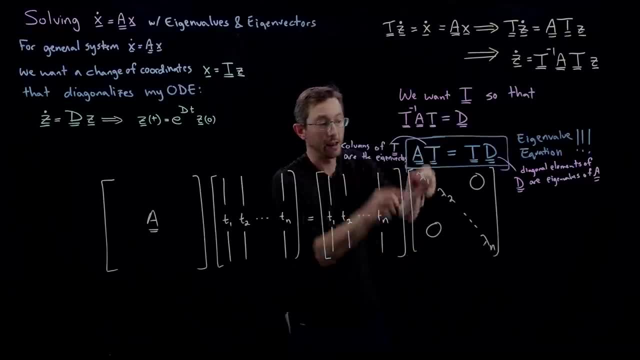 what I do is I take the first column of D and I kind of knock it over on its side and multiply it by every row of T. That's my first column. Then I take the second column of D, I knock it over on its side. 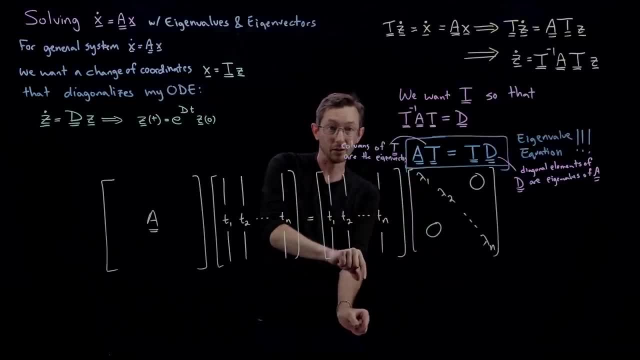 and I multiply it by all of the rows of T. That's my second column, And so on and so forth. But if you take, let's say this, lambda 2, you know this column here- and I knock it over on its side and multiply it, 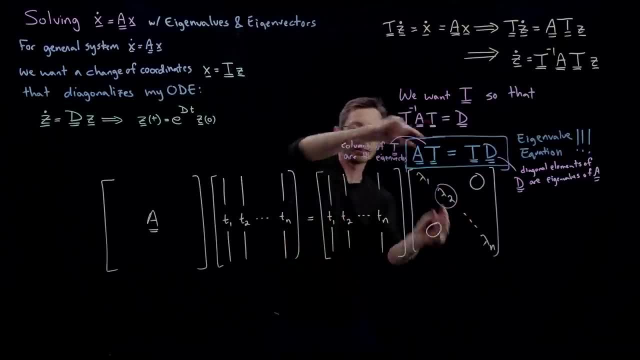 because it's zeros. everywhere else it's only going to multiply the T2 eigenvector. So this is a very useful property of this diagonal matrix. This literally is going to equal lambda 1, T1, that vector, Lambda 2, T2, that vector. 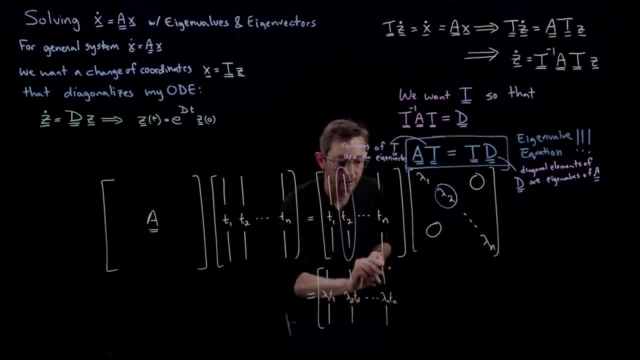 Dot, dot, dot. lambda N TN That vector. Okay, And so what we're basically going to find is that A times T1 is going to equal lambda 1, T1.. A times T2, the second column of this product. 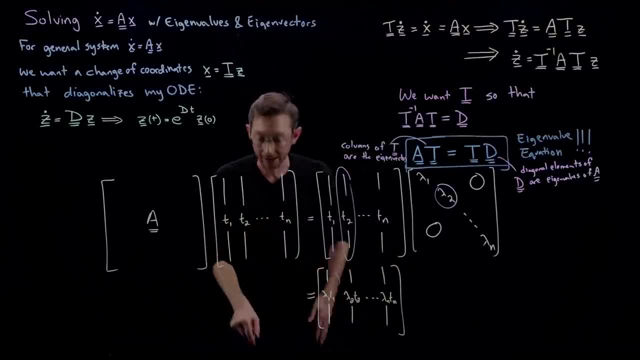 is going to equal lambda 2, T2, and so on and so forth. I'm going to get a bunch of equations that look like A times T equals lambda times T. Okay, Like for the k-th eigenvector and the k-th. 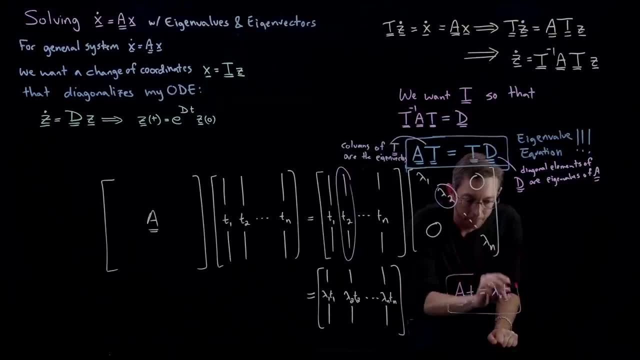 eigenvalue. this is going to be true. Okay, So you can write it in this matrix system of equations, or you can write it for a specific eigenvector, T, or eigenvalue lambda. Now, here, Tk is just a single eigenvector. 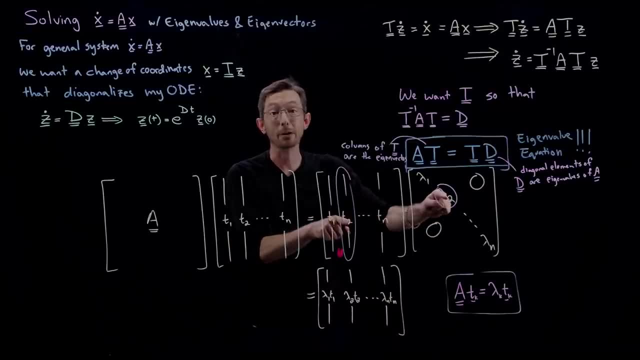 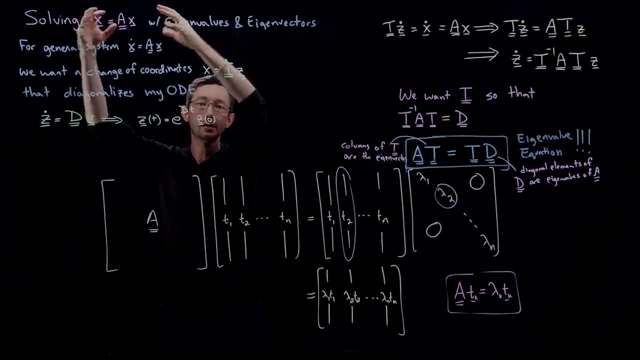 corresponding to that particular eigenvalue. These come in pairs, is what I'm trying to say. Okay, let's take a big step back. We want to solve these systems Generically. they are not going to be diagonal. We know that we like diagonal. 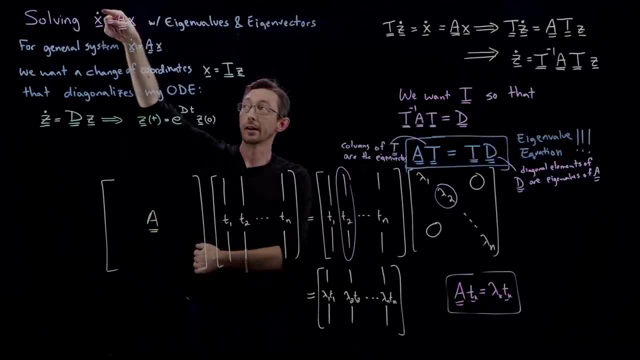 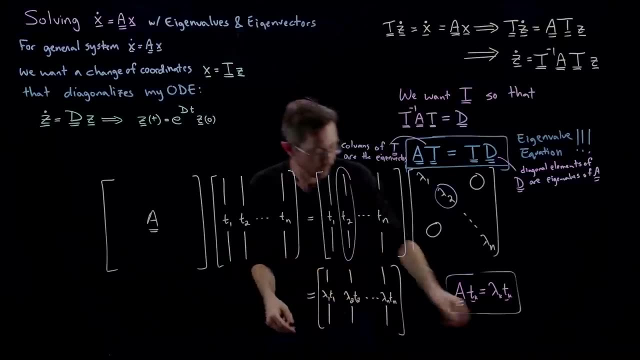 We know that we like diagonal systems because they're easy to solve, but generically they're not going to be diagonal. So we try to find a coordinate transformation T, a matrix T that can map me into a new coordinate system, Like literally, you know. 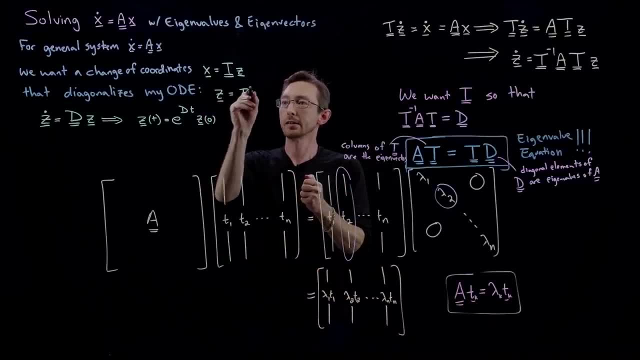 Z is going to equal T, inverse of X. So I can go from X to this new coordinate system, Z, so that Z has diagonal decoupled dynamics. So it's easy to solve my dynamics in Z. Now if I go through some algebra. 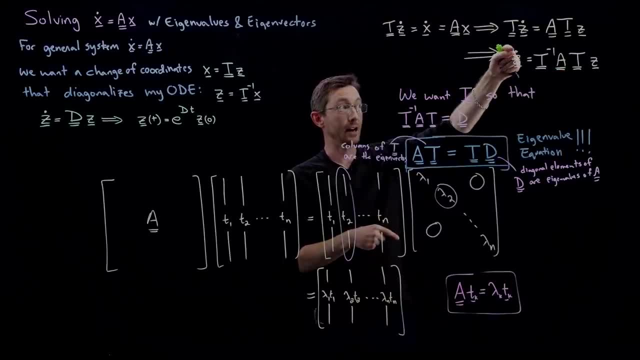 we find that This is the condition. So if Z dot, these are the dynamics in my Z coordinates, And so if I want these to be diagonal, then this has to be true And I can rewrite that in terms of my eigenvalue equation. 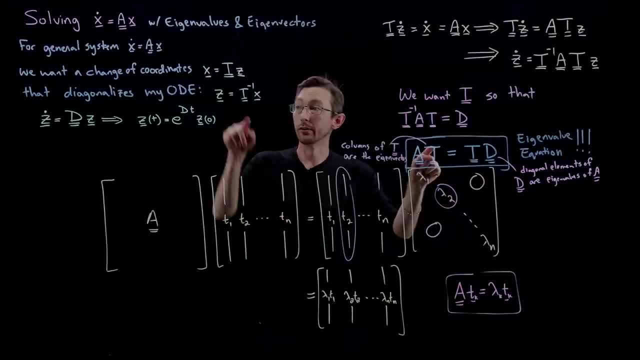 So this is the equation I solve to get that eigenvector coordinate transformation T that diagonalizes my matrix A, And given that we're going to be able to solve generic systems that are really nasty in terms of easy, easy, easy linear algebra, 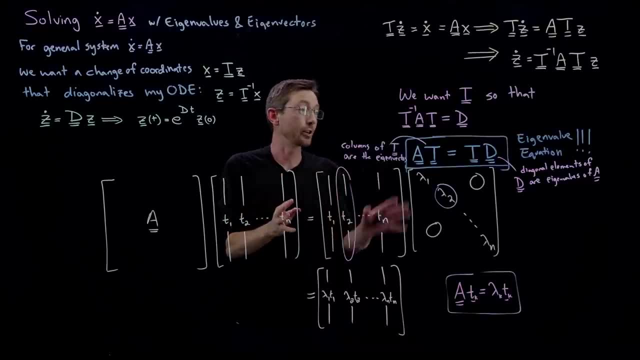 Okay, And that's all coming up. next, In the next lecture, I'm going to show you how do you actually compute eigenvalues and eigenvectors, And in the lecture after that, I'm going to show you how do you use that. 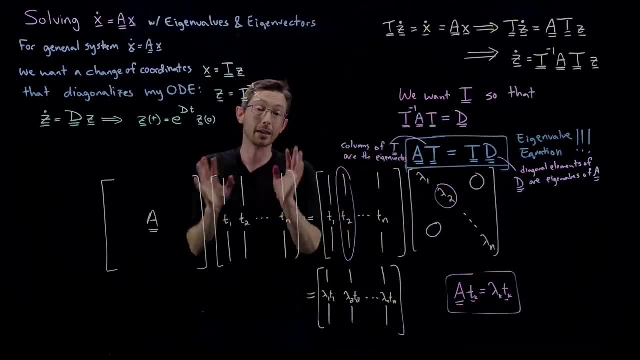 to actually solve these differential equations that we want. All right, Thank you.